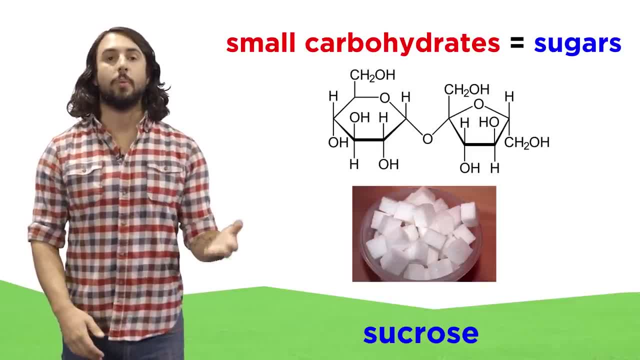 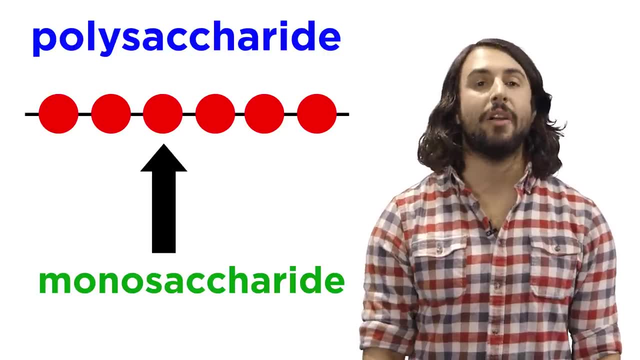 like glucose or sucrose, which is the sugar that we commonly refer to as simply sugar. Let's learn about monosaccharides first. These are the monomeric units that polymerize to form polysaccharides. We can name these according to the number of monosaccharides in the body and the number 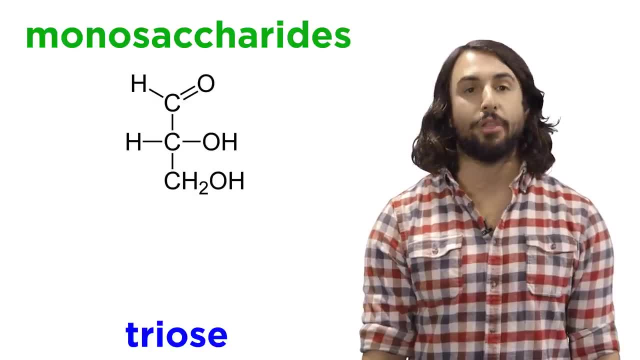 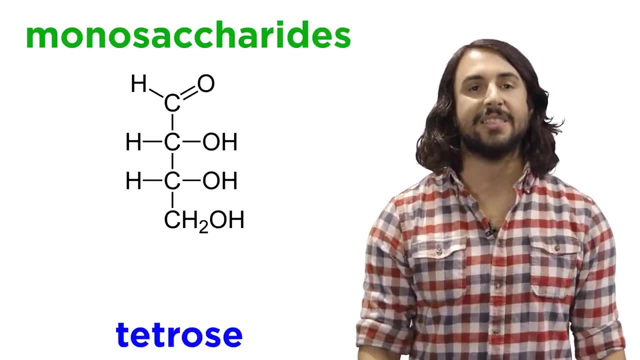 of carbon atoms they have, which will be between three and six. So a three-carbon monosaccharide would be a triose. If it has four carbon atoms, it's a tetrose. Five carbons would be a pentose. 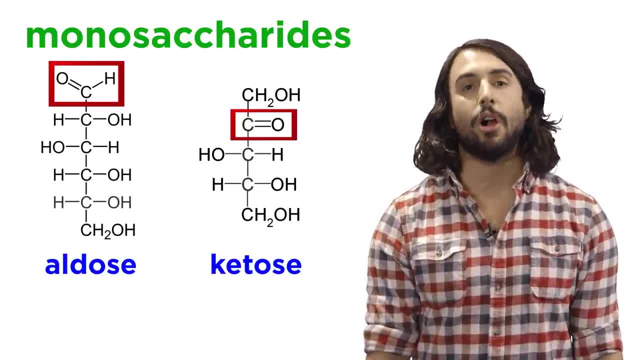 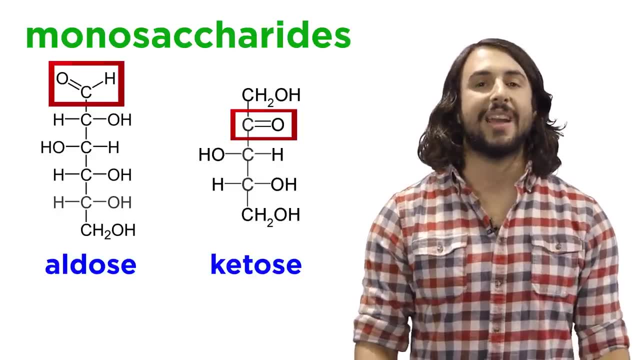 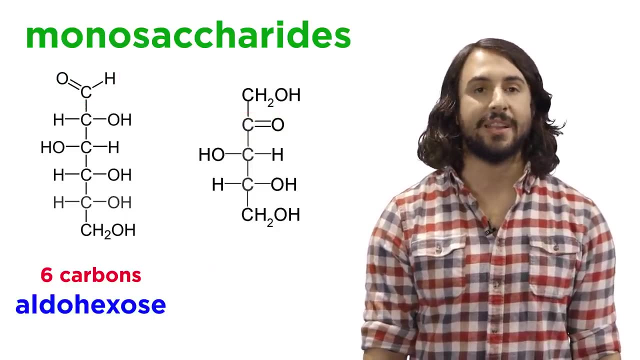 and six would be a hexose. In addition, all carbohydrates will have either an aldehyde or a ketone functional group in the molecule, so we would refer to those as an aldose or a ketose respectively. Combining these conventions, we could refer to this monosaccharide as an aldohexose, and. 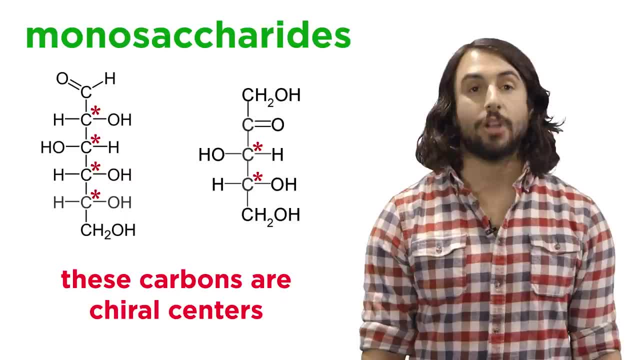 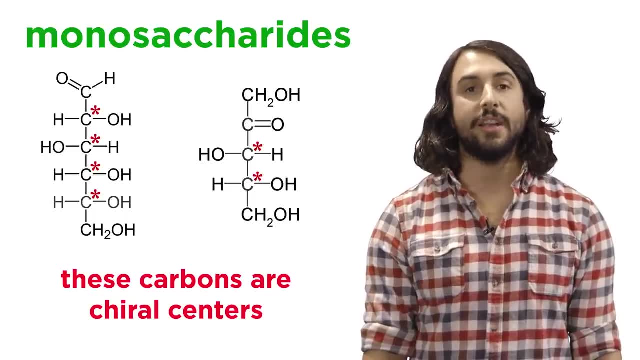 this one as a ketopentose. Each of these carbons, the ones that bear both a hydrogen and a hydroxyl, will be a chiral center, and the convention for drawing linear monosaccharides is to use Fischer projections. When we look at these, it is important to understand that. 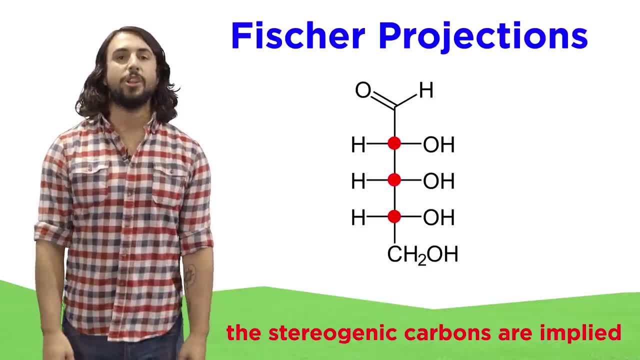 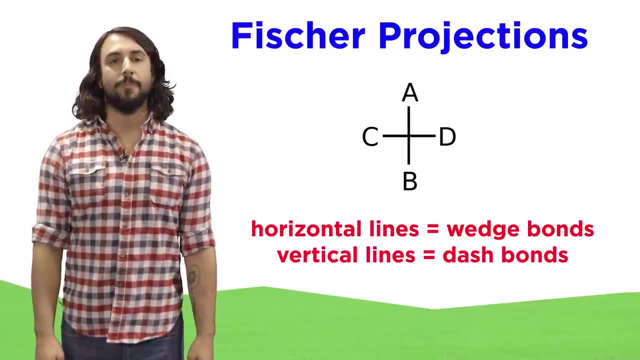 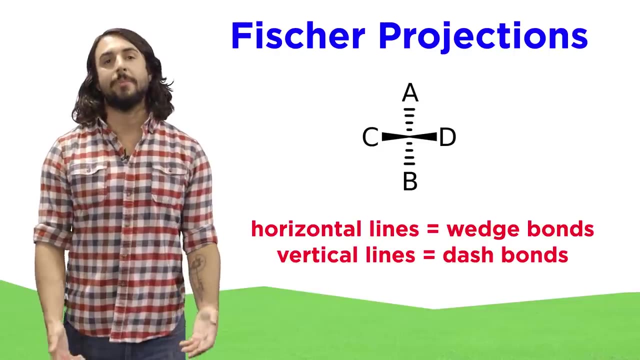 each vertex is a stereogenic carbon and we show the hydrogens and hydroxyls on either side With Fischer projections. horizontal lines are implied to be wedge bonds and the vertical lines are implied to be dash bonds. To remember this, just imagine a bowtie on each carbon. 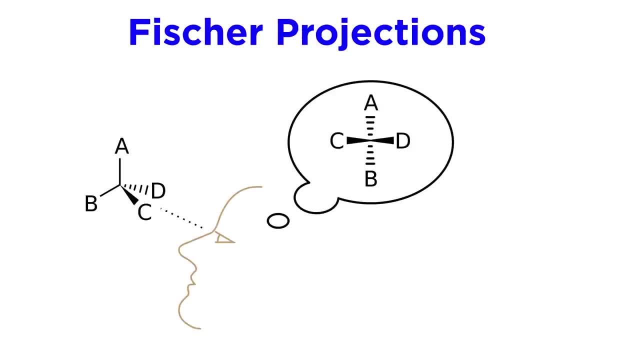 like it's going to the chemistry prom. Fischer projections are just a different way of visualizing a molecule, which we can see if we draw this molecule in line notation and view it from the side. The Fischer projection is what we would see if we were in the plane of the screen. 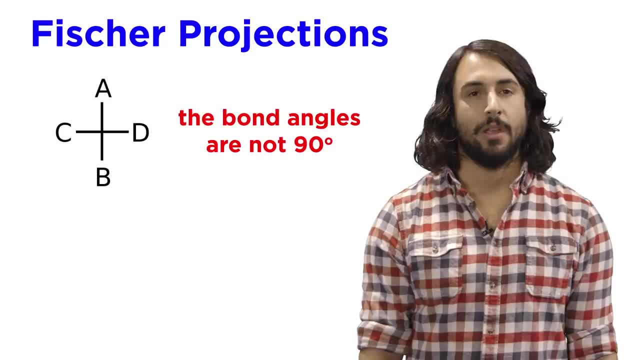 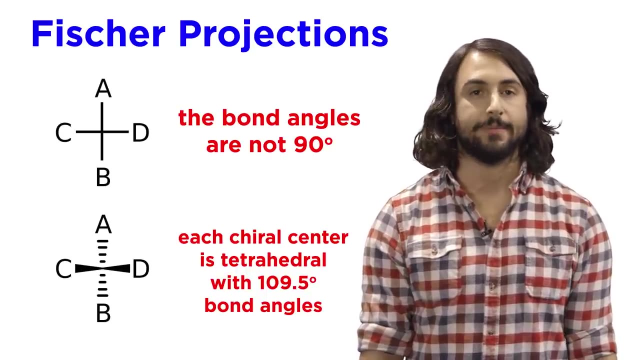 looking directly at the chiral center. However we choose to view it, it's important to realize that Fischer projections do not imply a flat molecule with 90 degree bond angles. These carbons are still tetrahedral. we just save time by drawing sugars this way When we draw. 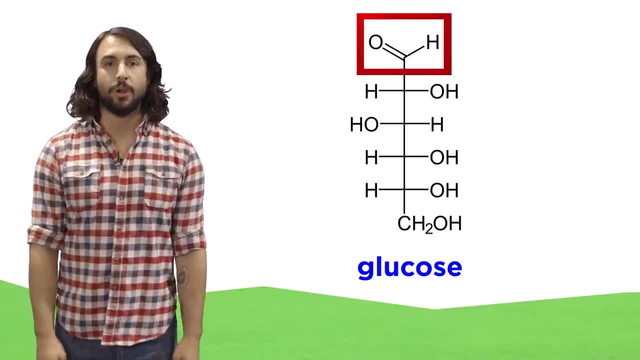 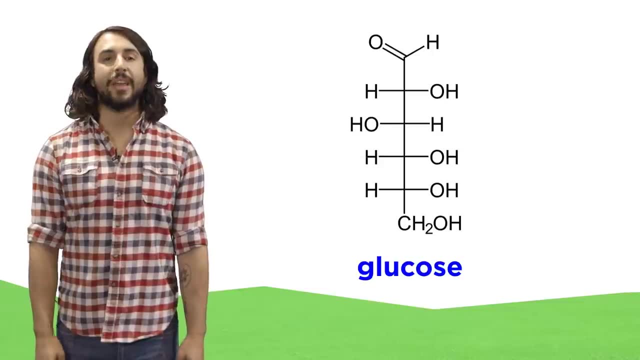 linear monosaccharides, we always put the aldehyde, or ketone, at the top and draw the rest of the molecule downwards. and we report the stereochemistry of the molecule by looking at the chiral center at the bottom, furthest away from the carbonyl. If on this carbon 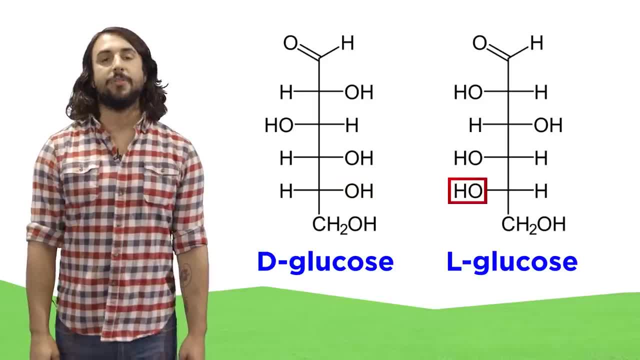 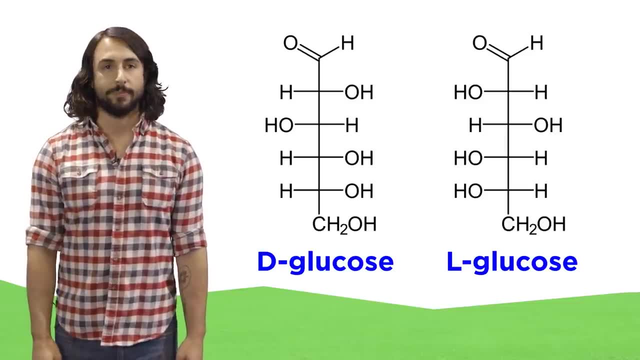 the hydroxyl points right, it's a D-sugar. If it points left, it's an L-sugar. So we would call this D-glucose and this would be L-glucose. This terminology is a bit more outdated than the R and S we use to assign absolute configuration. but the convention 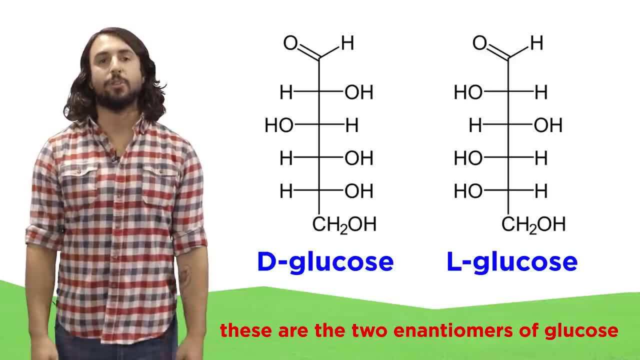 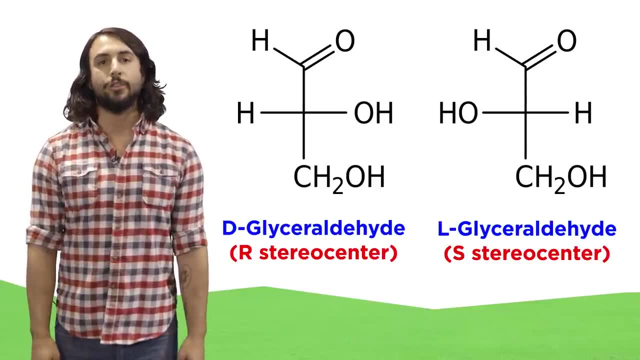 has stuck around and it remains the way that we differentiate between enantiomers of sugar molecules. We got this from glyceraldehyde, the simplest sugar, and an aldo triose. This has only one chiral center and we developed D and L terminology according to the two enantiomers of this molecule. 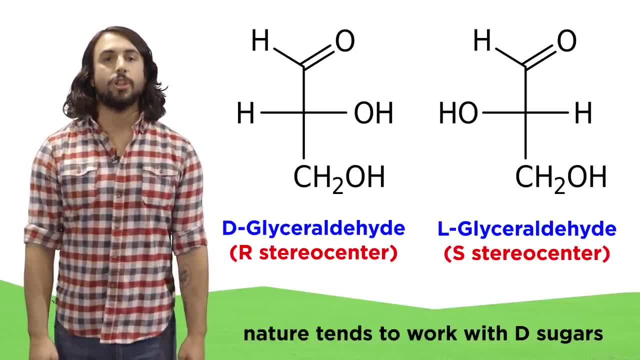 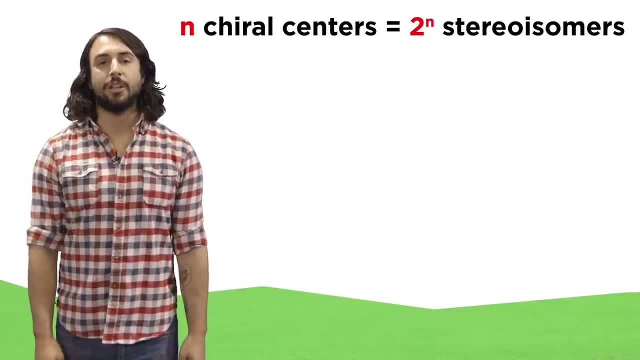 For some reason, nature has selected to work with D-sugars, so, unless otherwise stated, we can assume that we are talking about D-sugars. Let's also note that, since a molecule with N chiral centers has two to the N stereoisomers. 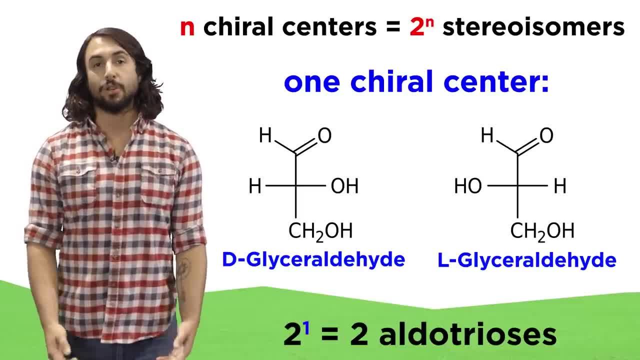 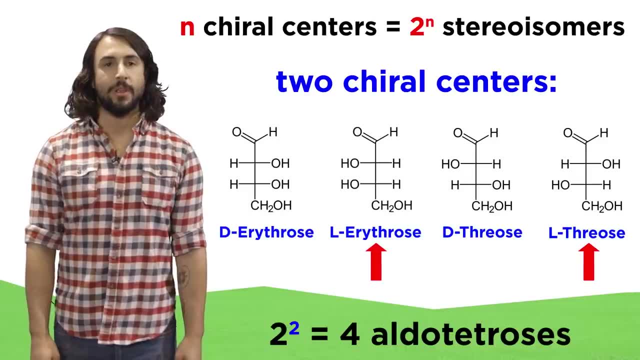 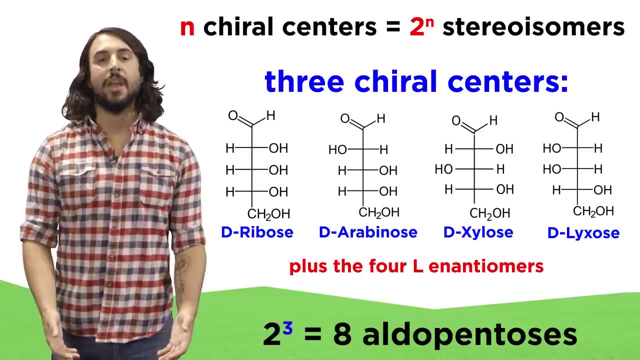 there are two aldo trioses, the two glyceraldehydes, since there is only one chiral center on the molecule. there are four aldo tetroses, these two and their L enantiomers. there are eight aldo pentoses- these four and their L enantiomers, because of the three stereocenters and a. 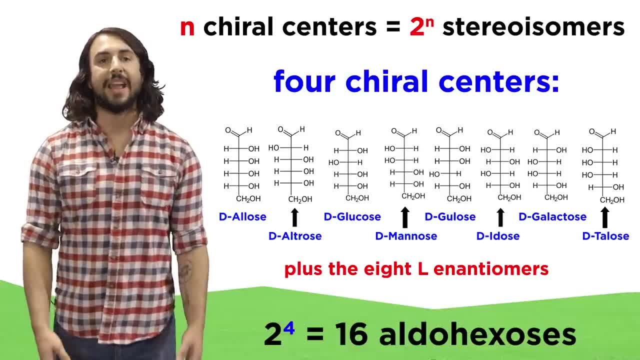 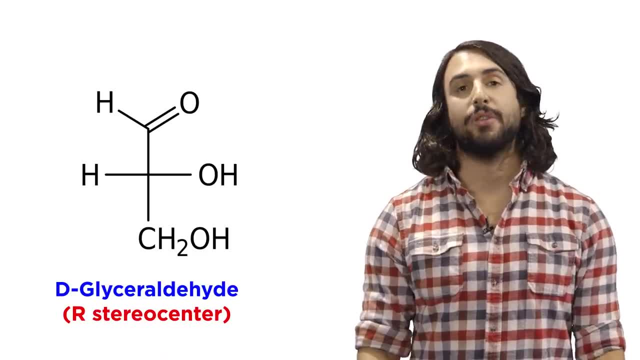 total of sixteen aldo hexoses. these eight and their L enantiomers. These differ only in the stereochemistry of these chiral centers. Lastly, with Fischer projections, let's look at the L enantiomers, For example. if you 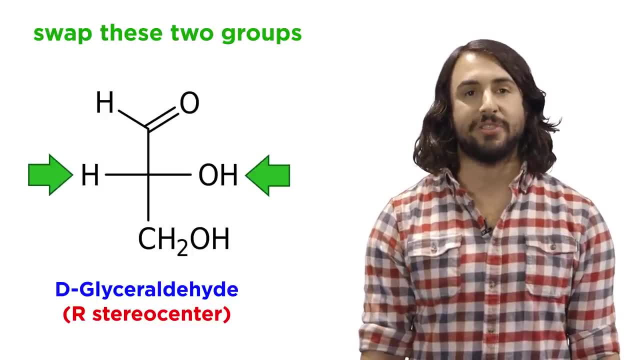 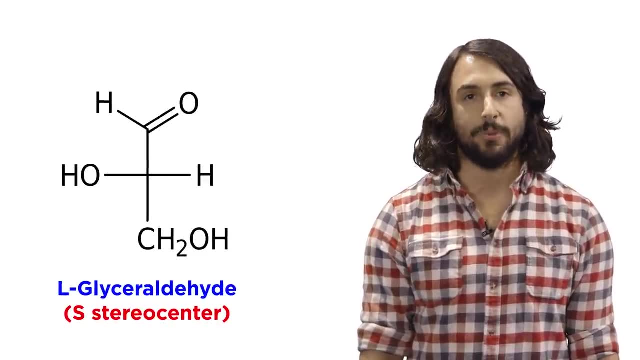 have two aldo pentoses, these two and their L enantiomers, because of the three stereocenters. let's be sure to understand that swapping the position of two groups on a chiral center results in the inversion of that stereocenter and a totally different molecule. and while 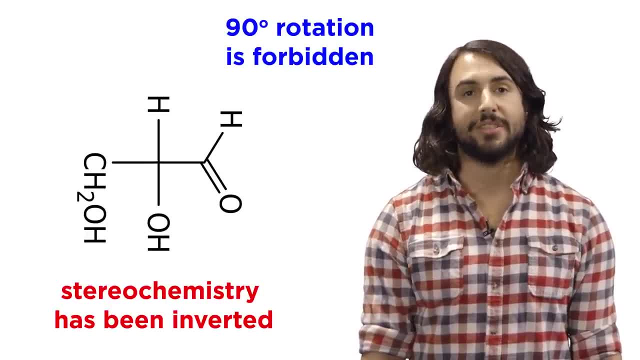 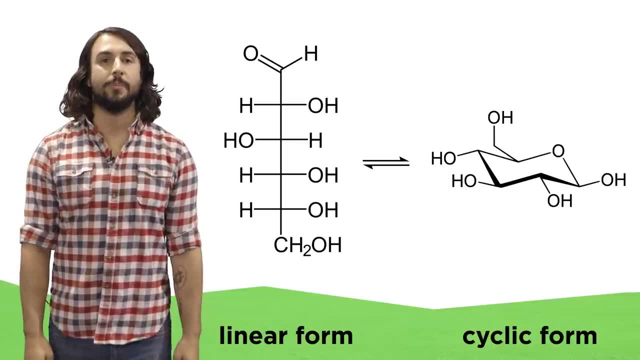 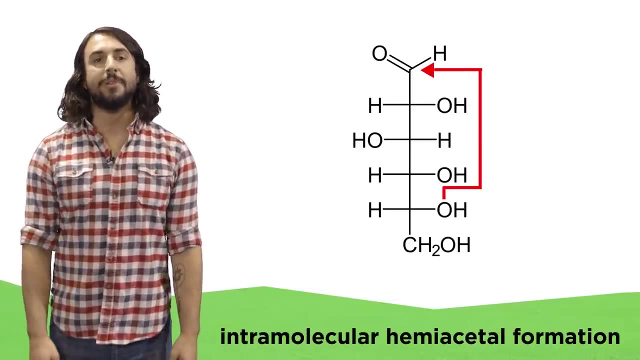 90 degree rotations are forbidden because they invert stereochemistry. 180 degree rotations are allowed. Monosaccharides exist in an equilibrium between a linear and a cyclic form, with the cyclic form being highly preferred. They cyclize by an intramolecular hemiacetal formation. 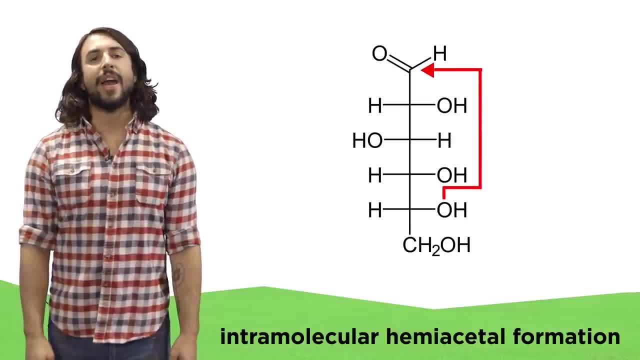 A mechanism we learned in organic chemistry. We know that when hemiacetals form, it's because an alcohol attacks an aldehyde or ketone. In this case, it's an intramolecular cyclization, because the hydroxyl group and the carbonyl 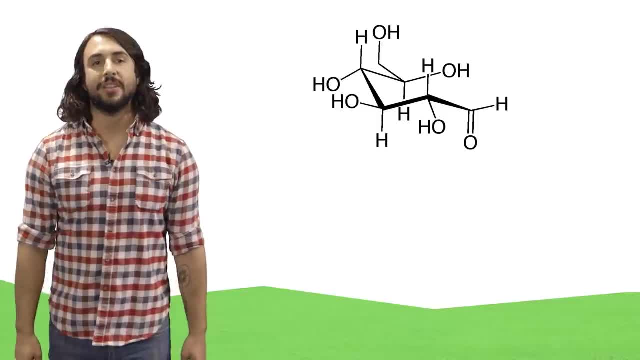 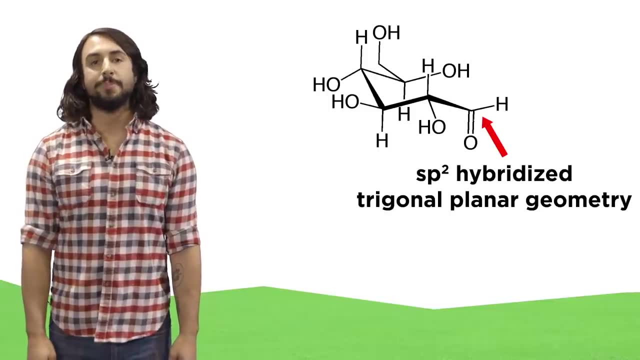 are on the same compound. Now let's orient this linear molecule in a way that we can see the cyclization take place. We know that carbonyl carbons are sp2 hybridized and therefore exhibit planar gyroscope. We know that carbonyl carbons are sp2 hybridized and therefore exhibit planar gyroscope. 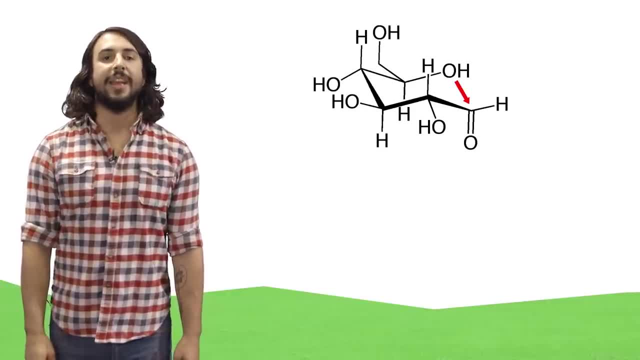 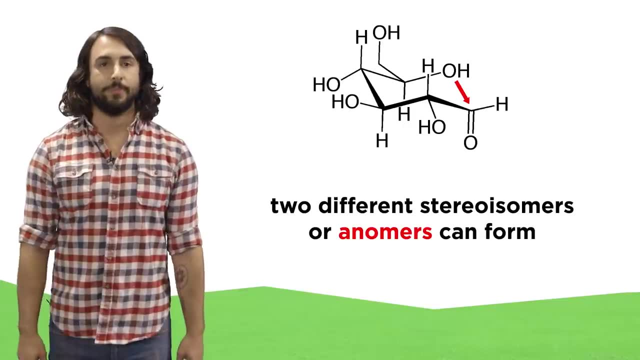 We know that carbonyl carbons are sp2 hybridized and therefore exhibit planar gyroscope. So when the hydroxyl attacks the carbonyl, it can do so from either side, thus generating two different stereoisomers, which are called anemers. 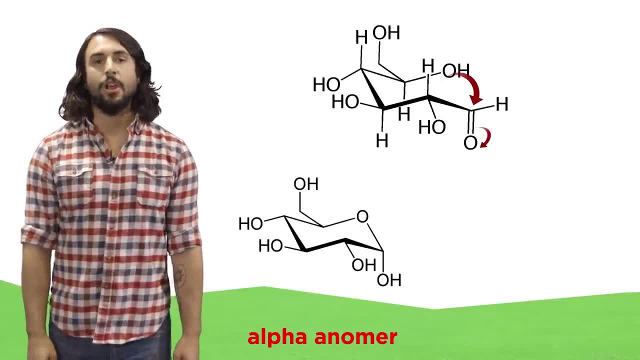 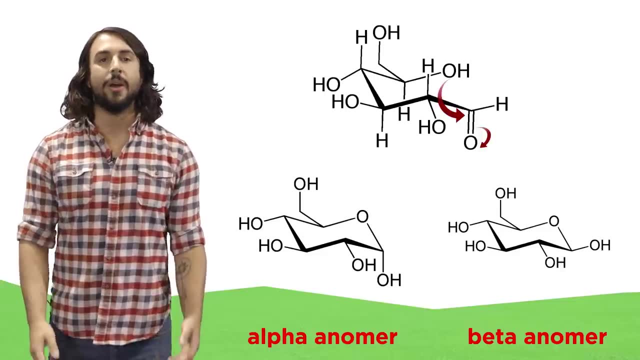 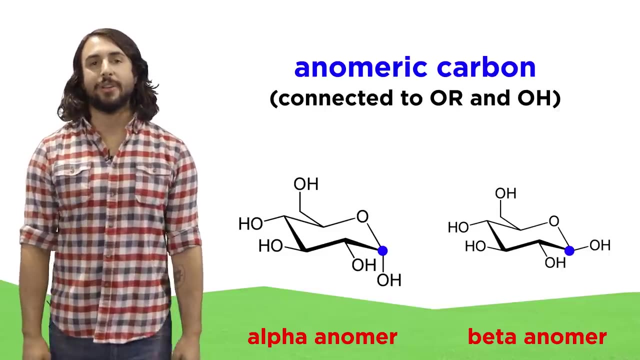 It can either attack from this side, pushing the new hydroxyl down, resulting in the alpha anemer, or it can attack from this side, pushing the new hydroxyl up, resulting in the beta anemer. That makes the resulting hemiacetal carbon the anameric carbon. because we can either 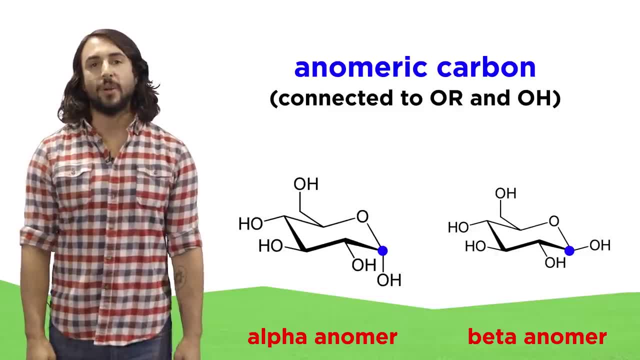 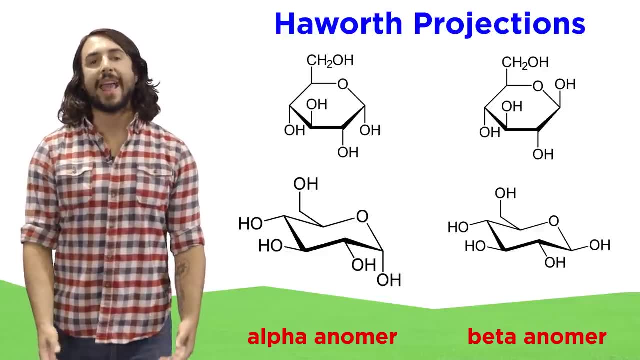 get the alpha anemer by moving the hydroxyl up or the beta-anomer, depending on which side the hydroxyl attacks from. when we draw cyclic monosaccharides, we sometimes use Hayworth projections. with these we look at the ring from the edge, meaning. 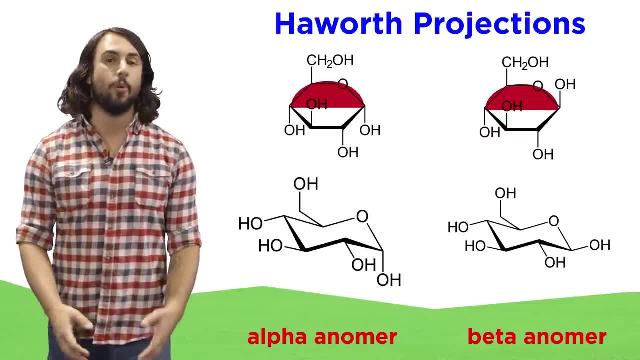 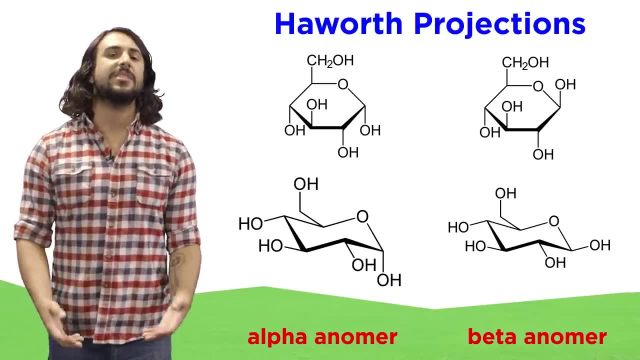 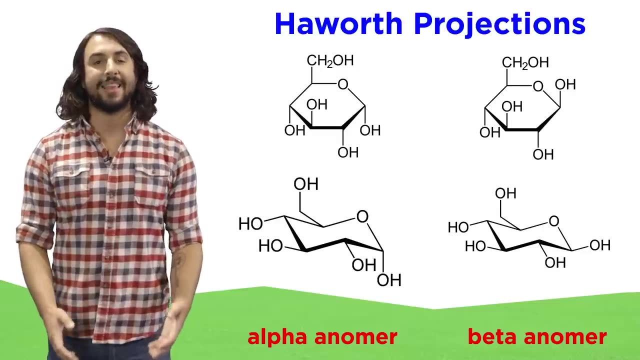 this part of the ring is closer to us and this part is further away from us, and we show the functional groups projecting straight up and straight down. this does not accurately display the true geometry of the molecule, because we know six-membered rings like these. 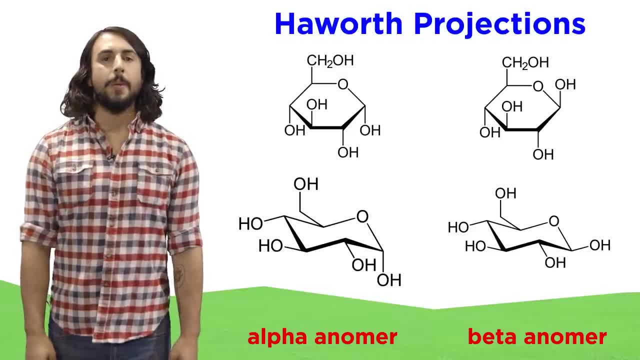 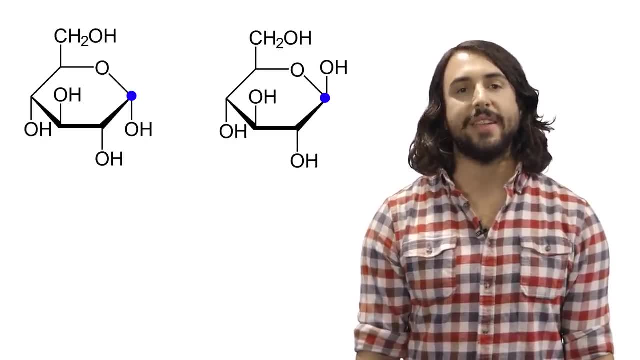 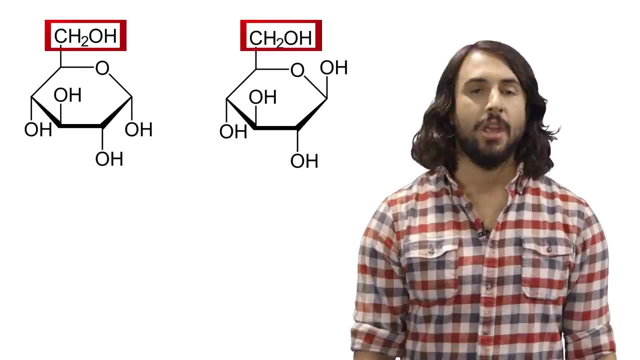 prefer to be in a chair conformation, but Hayworth projections have other practical uses. when we draw these, the convention is to place the anomeric carbon on the right and the CH2OH on the other side of the ring, pointing up if 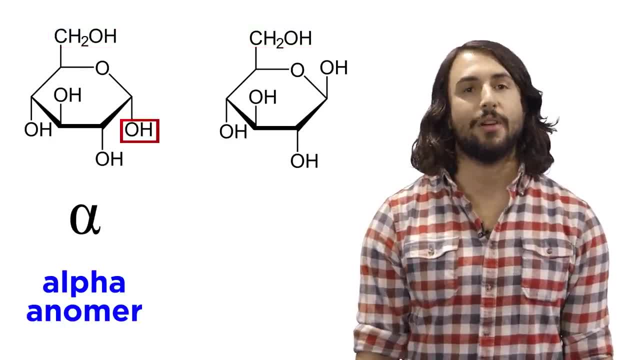 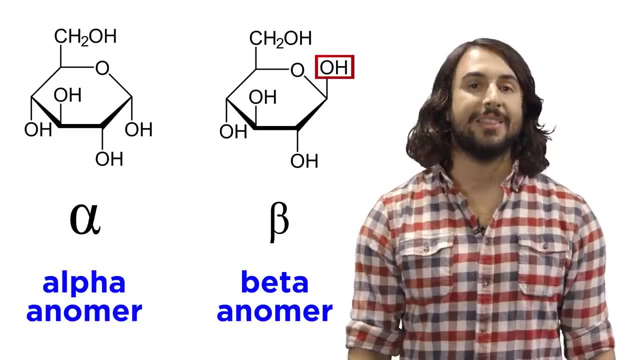 the new hydroxyl group that was generated during hemiacetal formation points down and is trans, to this group, we have the alpha-anomer, and if it is pointing up cis to this group, we have the beta-anomer. if a cyclic monosaccharide has a 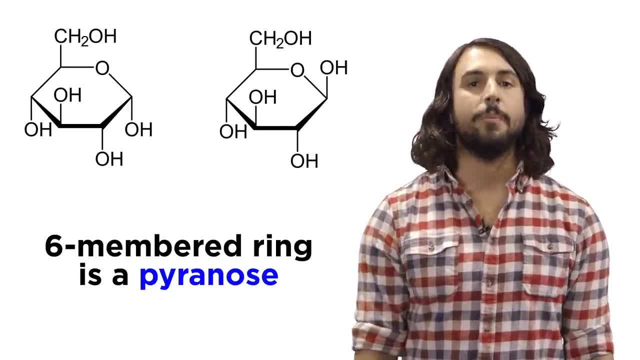 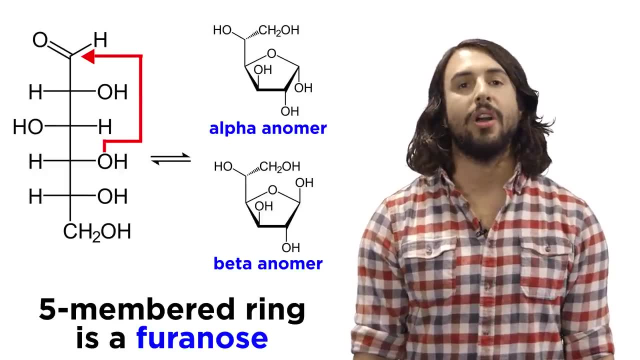 six-membered ring- we will call it a pyrinose. but sometimes the hydroxyl uncarbon-4 can do the attacking, resulting in a five-membered ring, which we will call a furinose. rings smaller than this are unlikely to form due to.